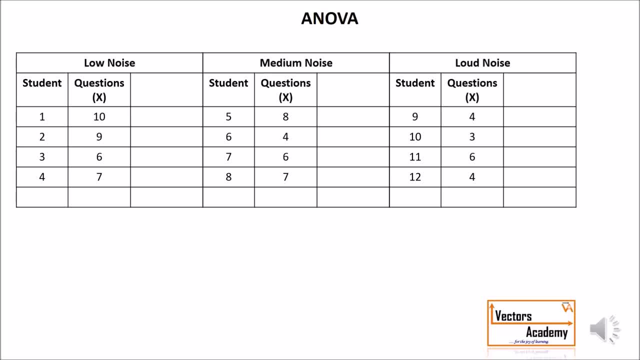 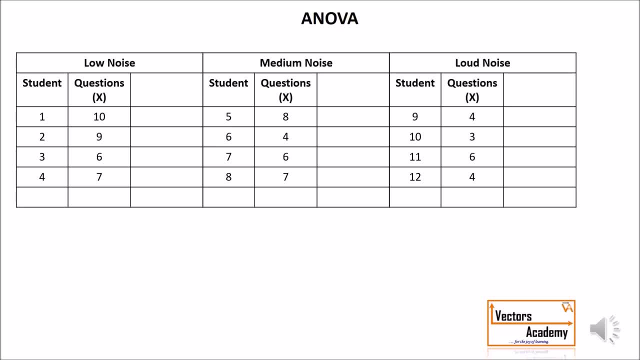 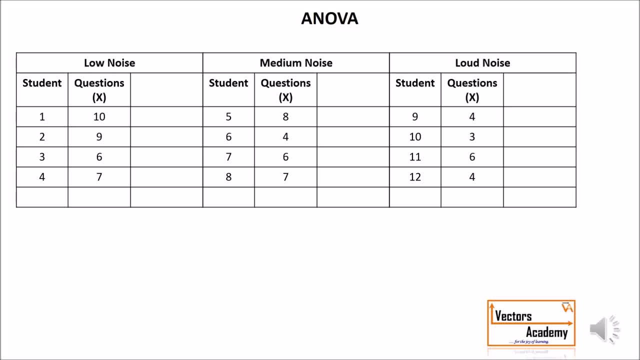 This time the variable noise. we cannot rate that noise, So we have rated it into three different categories. If we could rate that noise scale of 1 to 10, we could actually use the Carl Pearson's coefficient of correlation to find out what is the relation between them. 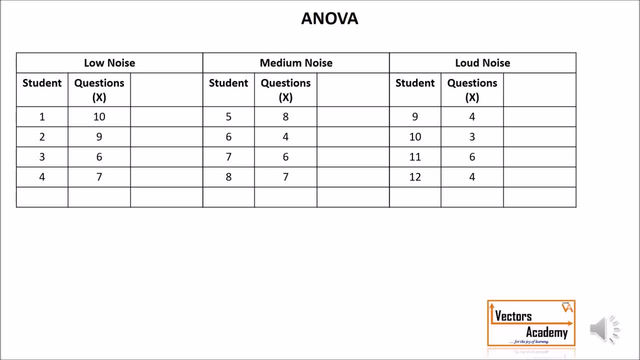 But in this we just have one variable, that is the number of questions, whereas noise cannot be rated. So what we do is we first name the questions as X. X represents the number of questions solved. So we make a new column that is X square, for all the three voices, noises. 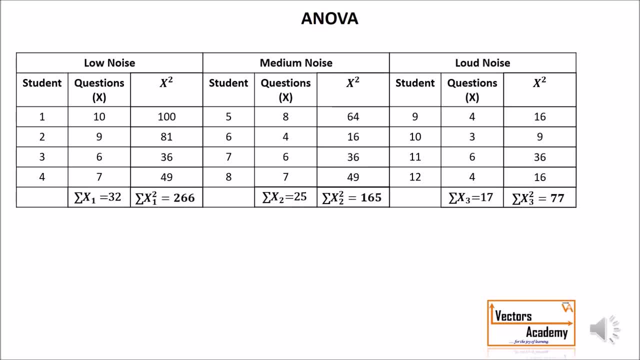 And we take the total of all these columns. So what we need to do is to just note these total, which are required to start our calculation. Now we'll start with our analysis. The first thing we need to calculate is the correction term. 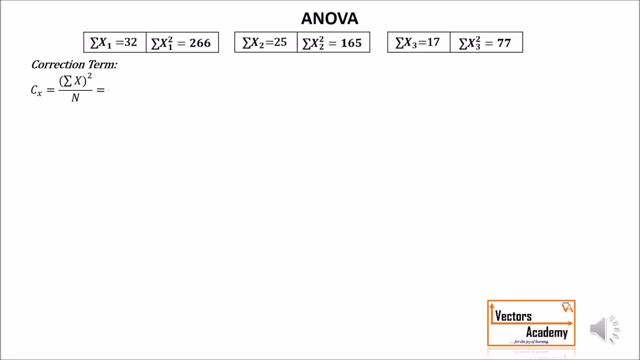 Now the correction term is given by the formula: summation of X. the whole square upon N. N represents the number of students which we have. We have 12 different students, four in each category. So we'll get the answer: 32 plus 25 plus 17,. the whole square upon 12.. 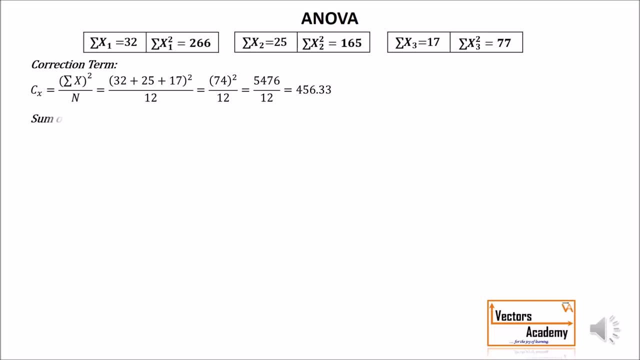 The answer comes to 456.33.. The next is sum of squares of total. Now, Summation of squares, addition of all these squares minus the correction term. So that is 226 plus 165 plus 77.. We have to add all these totals and subtract it from the correction term which we have calculated. 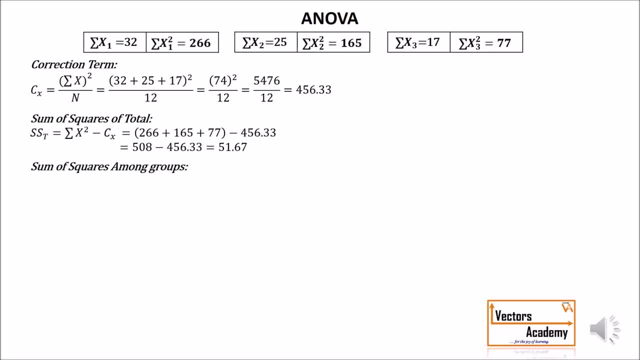 So that comes to 51.67.. Next is sum of squares among groups. That is given by the formula summation of x, the whole square divided by small n, minus the correction term. What is small n? Small n is the number of students in each category. 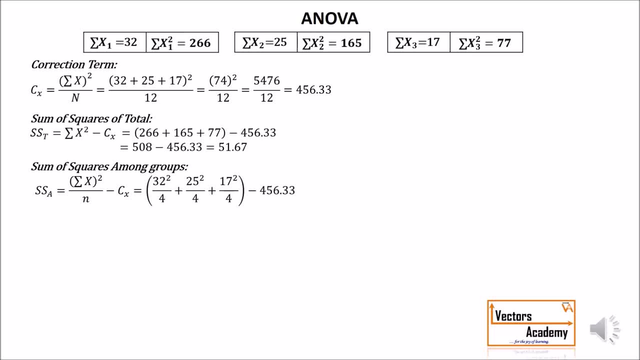 In each category we have 4 number of students. So what I will do is I will square 32 divided by 4.. Square 25, which is the total of all the questions in the medium noise divided by 4 students. In the same way for the loud noise as well. 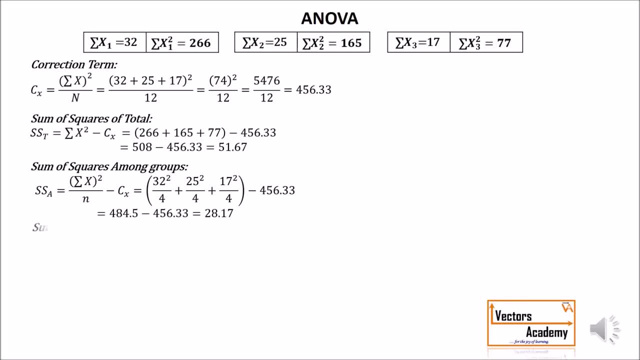 And we have to add all these fractions and subtract it with the correction term. So I will get this 28.17.. Next is sum of squares within groups. So both the terms we have calculated, sum of squares of total and sum of squares among groups. 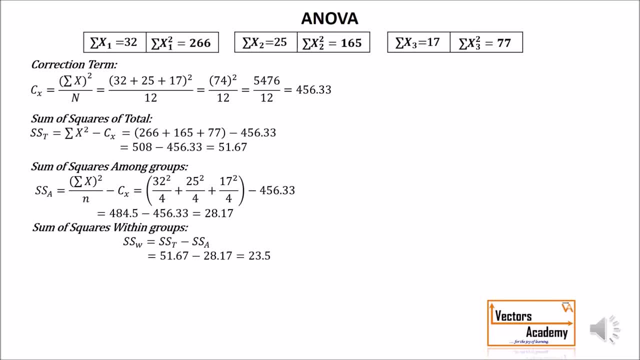 You have to subtract them and I will get the value of sum of squares within groups as 23.5.. Once you have calculated sum of squares, we now come to the mean of squares among groups. That is given by the formula sum of squares among groups divided by k minus 1.. 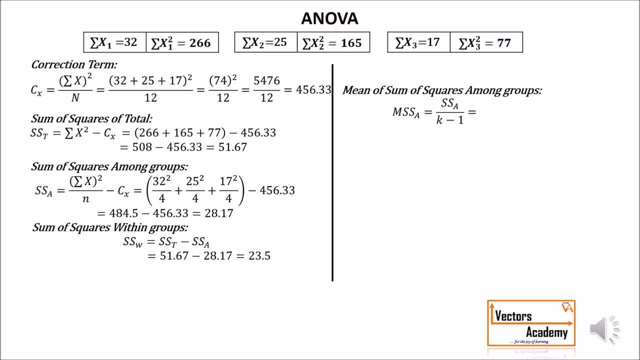 What is k? k is actually the number of categories, The categories of noise, which we have divided. There are 3 different categories, So the value of k is 3.. So the answer for the mean of sum of groups comes to 14.085.. 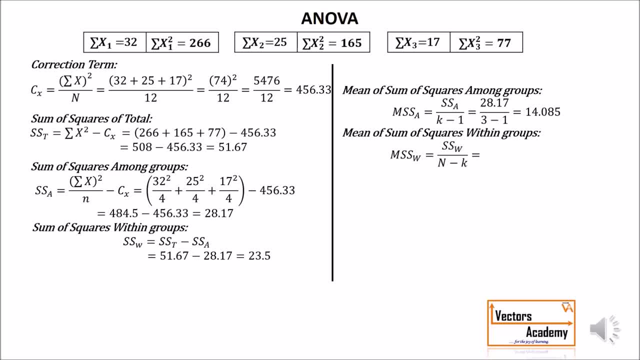 Next is mean of squares within groups. The formula is sum of squares within groups divided by n minus k. Remember, n is the total number of students and k is the different categories which we have. So the answer comes to 2.611.. And finally, we calculate our f. 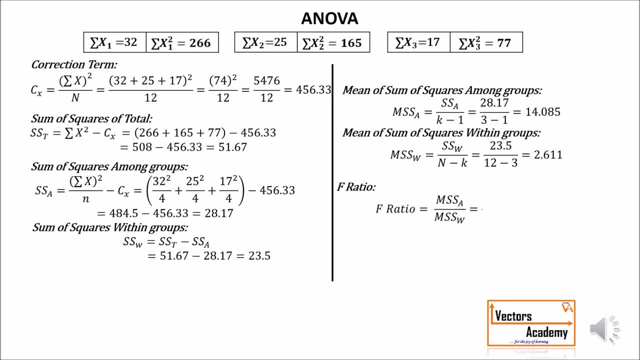 Ratio, That is Fisher's ratio. That is the division of mean of sum of squares among groups. divided by mean of sum of squares within groups, That comes to 5.394.. Now, once you have calculated all these, we will summarize what we have all calculated. 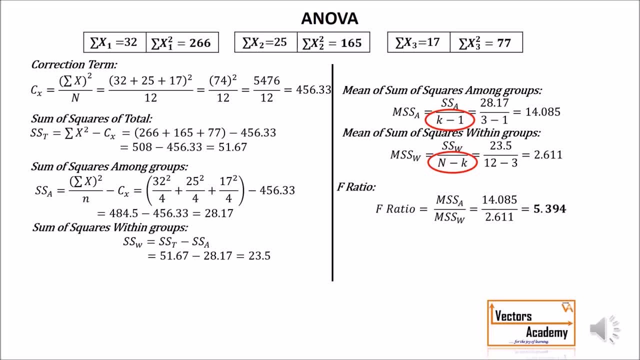 We need to also notice these two terms, That is, k minus 1 and n minus k. These are actually called as degrees of freedom. k minus 1 is the degree of freedom among groups, Whereas n minus k is the degrees of freedom within groups. 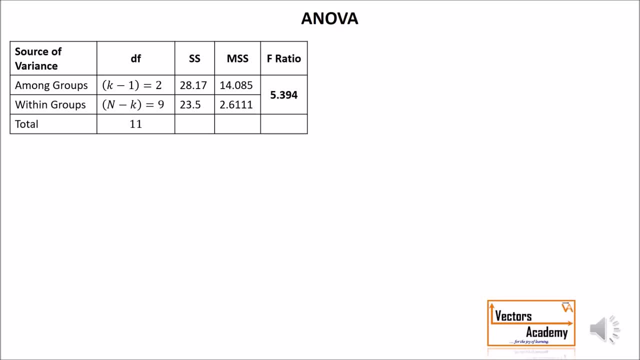 Now we will summarize whatever we have calculated so far in a table. Now the value of f ratio. That will actually tell us what significant level we can confidently say that there is a correlation between noise and the number of questions solved. So we will put on two hypotheses. 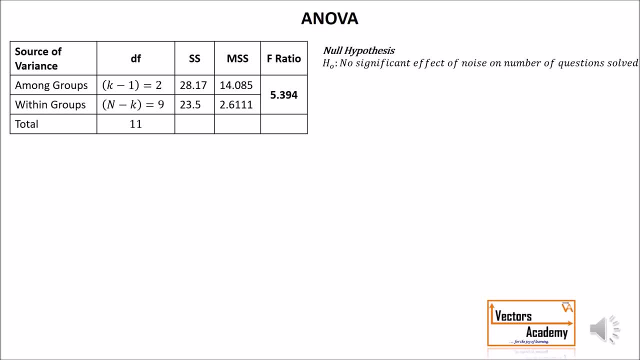 One is a null hypothesis, which indicates that there is no correlation between these two variables, and the other is an alternative hypothesis, which represents that there is a correlation between these two. Now we have a table for the f-ratio which will be given to you. 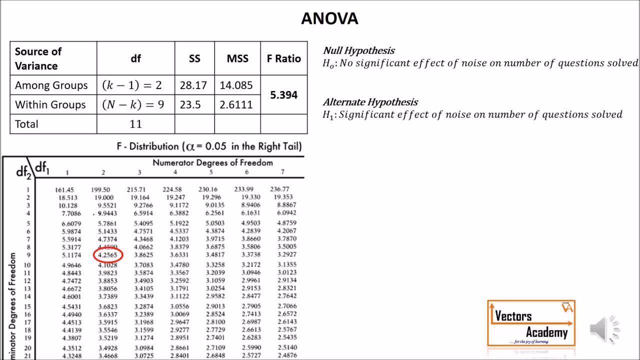 Now just take a look at this value. Now. this value is found out by the degrees of freedom, Right, Right. So here the degree of freedom among groups is 2 and the degree of freedom within groups is 9.. So in the table we have to find out the value which represents 2 in the upper row and 9 in the left side column. 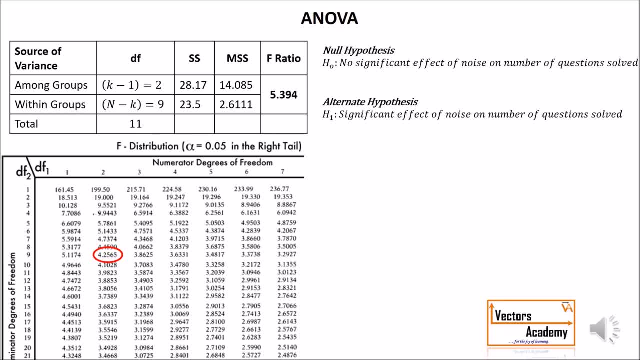 So the value is 4.2565.. Now we have to compare this value with our f-ratio. You can see the value which we have calculated is quite more Right. It is more than the required value. So what we do is we reject the null hypothesis and accept the alternative hypothesis, which is: there is a correlation. 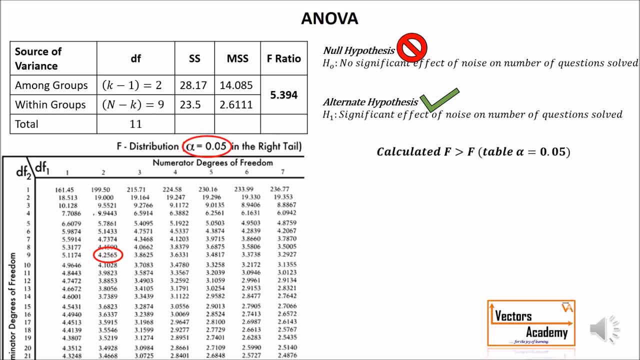 Now in the table this value alpha, that is 0.05. that represents what the error is. The error is 0.05.. So that means we have 0.95% confidence level. That is 95% confidence level That there is a significant error. 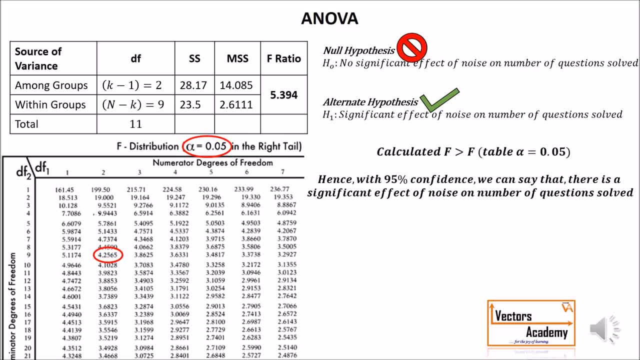 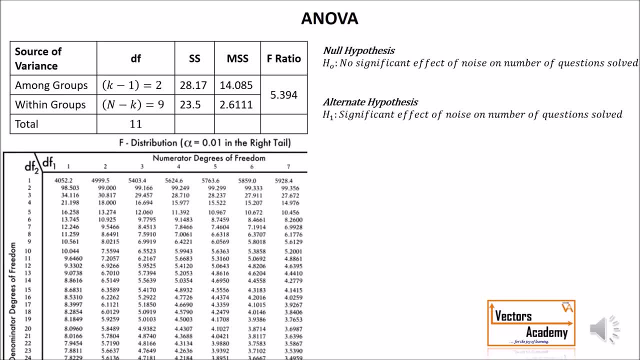 That there is a significant effect of noise on the number of questions solved. Okay, So in the same way there is another table that is for 0.01.. The value of alpha is 0.01.. So for that we need to get the values again.